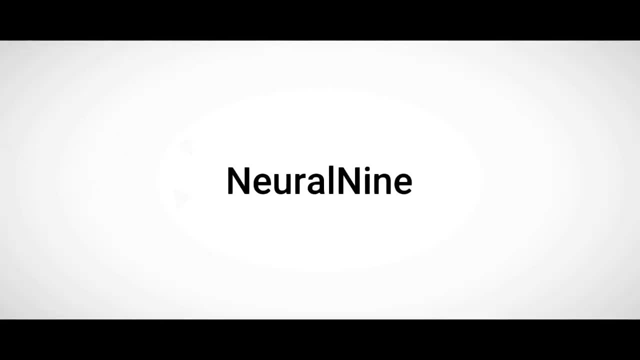 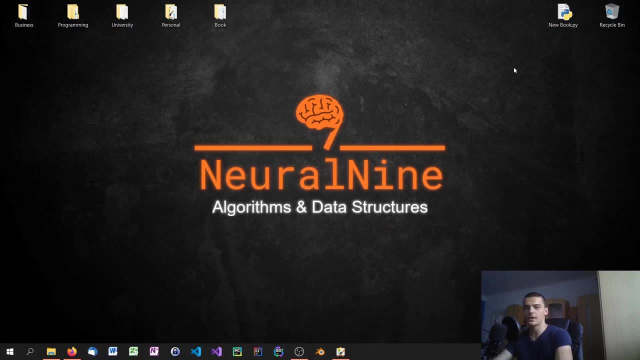 What is going on, guys? Welcome back to the algorithms and data structures tutorial series. In today's video, we're going to talk about greedy algorithms, and greedy algorithms are essentially just a category of algorithms that have certain characteristics, and in today's video we're going to briefly mention them. We're not going to talk about them too much in detail. 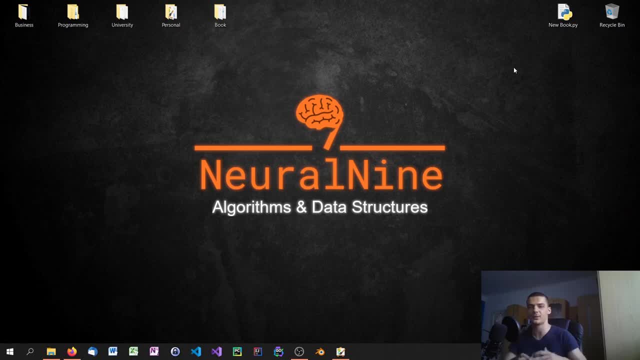 I just want you to have heard of them, which is why I'm making this video at this point in the series. I want you to know about greedy algorithms, what they are, what they look like. We're going to look at an example today so that you can see how greedy algorithms look, so that you can recognize. 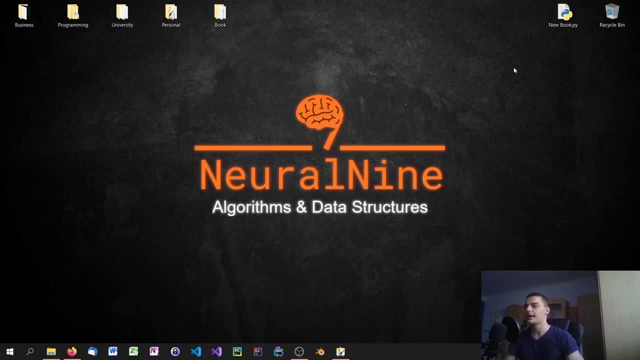 them in future videos. We're going to use some of them in the future and I also want you to see that sometimes they're very efficient, or you should use them in some cases, and sometimes they don't produce optimal results, So let us get right into it. So, in order to explain, 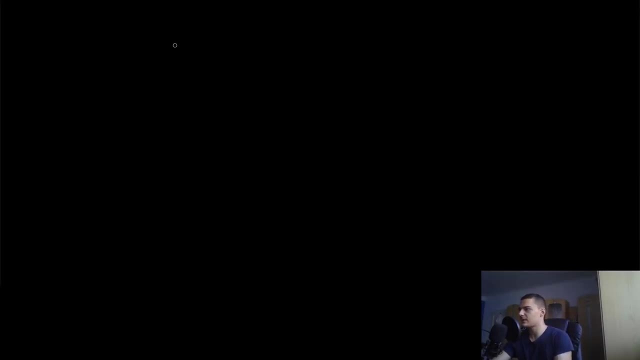 greedy algorithms. I'm going to use a very simple example. Let's say we have three types of coins, So we have one cent, we have five cents and we have ten cents. These are the types of coins that we can use, and we have an unlimited amount of those. So now the question is if I'm given a 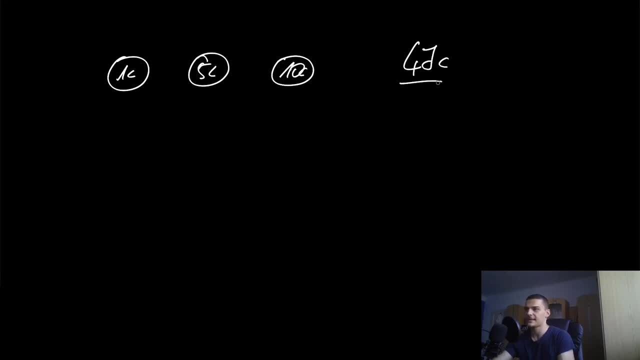 certain amount of cents, for example 47 cents, how can I find the optimal solution when the goal is to get to that amount? to give the person this amount of cents with the least amount of coins possible, with the smallest amount of coins possible. So, of course, if someone says I want 47, 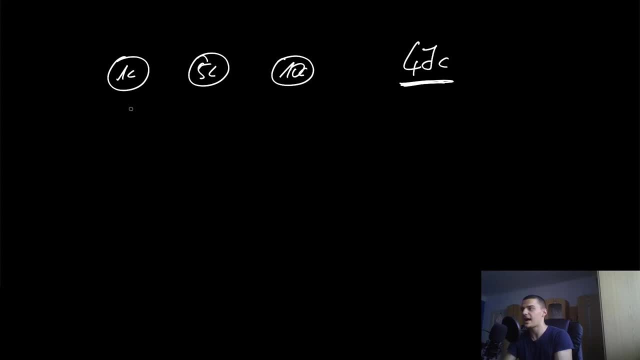 cents and I have an unlimited amount of all these coins. I can just go ahead and say, okay, I'll give you one cent 47 times, but then I end up with 47 coins, which is not an optimal result. And the question is: can we find an optimal solution Now to this problem? the optimal solution would be: 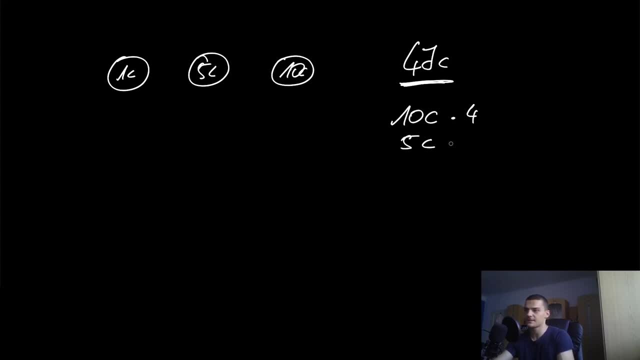 ten cents times four, five cents times one and one cent times four. So we end up with seven coins and a total of 47 cents. This is a very simple solution, an optimal solution, And the question now is not just: how can you solve this for a particular number, for example? 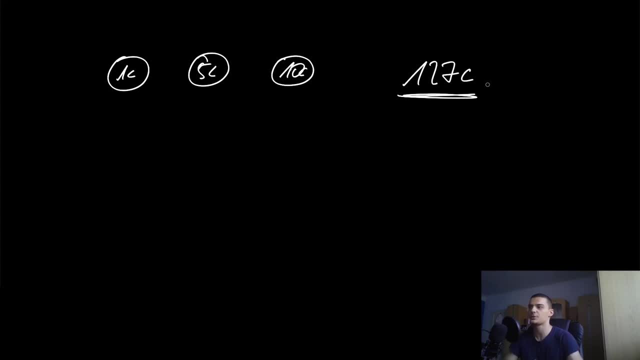 127 would be another number that we can choose. The question is: can you find an algorithm- and we don't need to write down the pseudocode- just by logical thinking? can you find an algorithm that always gives you the optimal solution? And it's not obvious that any algorithm that seems intuitive? 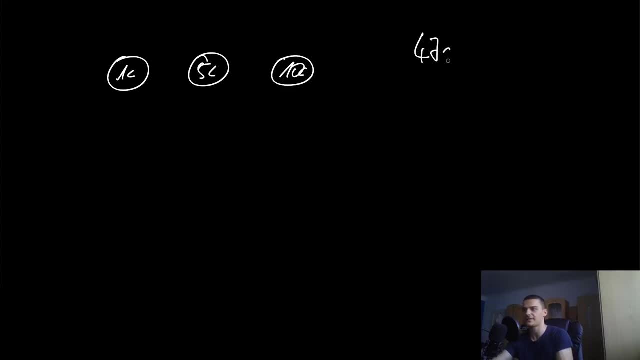 works here. So now, what we did in the first example here, with 47 cents, for example, is we just looked at: okay, what is the largest coin here? 10 cents. okay, how many times can I use 10 cents in order to get to 47? okay, I can use it four times so I end up with seven cents left and then I can use the five cents. 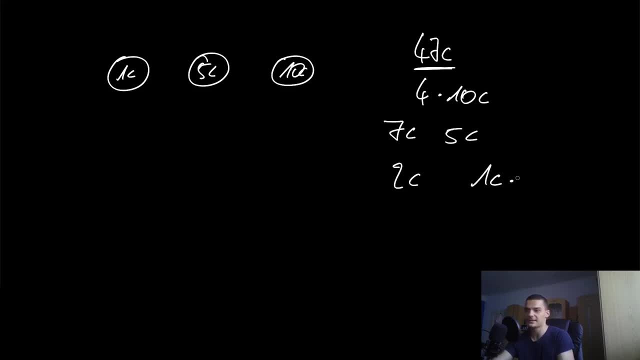 then I have two cents left, so I can just go ahead one cent times two. okay, Now what we're doing here is applying a so-called greedy algorithm, And in a, greedy algorithm is defined by always picking the solution, the local solution that seems the most beneficial. 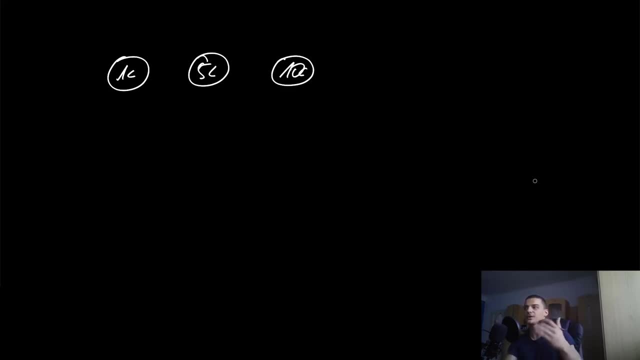 right now. So you're not looking long term, you're thinking: okay, what decreases the value of the of the price here? so we have 47 cents Decreasing 47 cents. the most, with one step is is done by subtracting 10 cents. right, It doesn't have to be the case that subtracting 10 cents is necessarily. 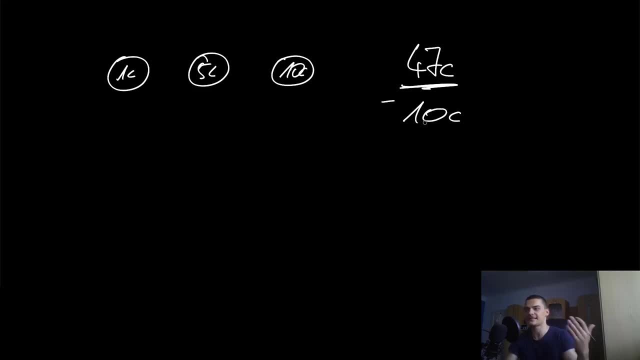 the best solution Long term. maybe if I subtract 10 cents now, it's going to be a problem later on. Now I can spoil the surprise for you. in this case, in this constellation, the greedy algorithm will always give us the best result. So actually doing this and picking the largest possible number will give. 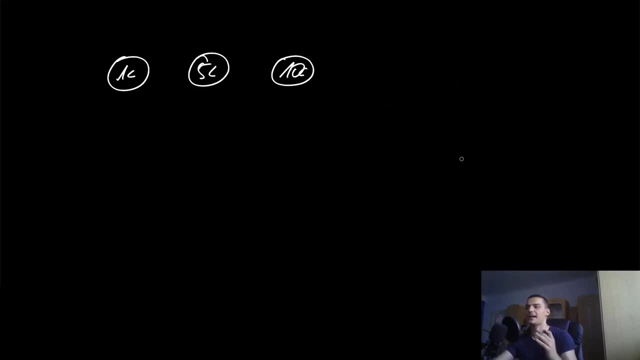 us the best results in this case. But this is what a greedy algorithm does. it looks at the value 51, for example, and asks: okay, how can I decrease this value the most with my next step? It doesn't ask the question of how can I decrease it in in the long run with the least amount of coins. 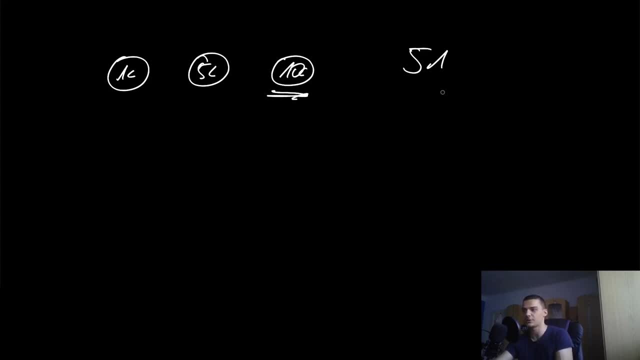 possible. It looks okay. which is the next value that I can choose to decrease this number the most? and the answer is the largest coin, and we do this as long as the largest coin still fits into the value, and then we choose the other coins. However, it is not always necessarily the case that a greedy 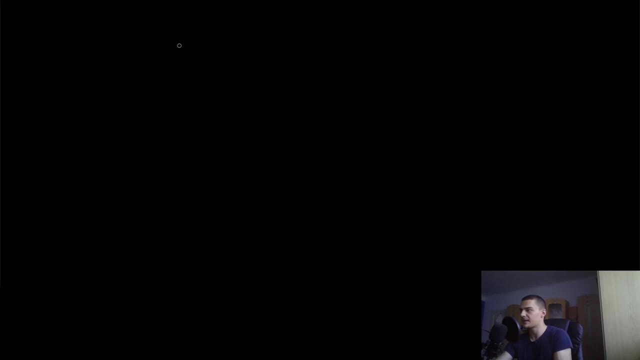 algorithm gives you the best result possible. For example, let's pick a different set of coins, So we have one cent, five cents and ten cents again, but then we can also add 20 cents and 25 cents. Now notice, I'm not picking any prime numbers or something. I'm not picking any super crazy numbers. 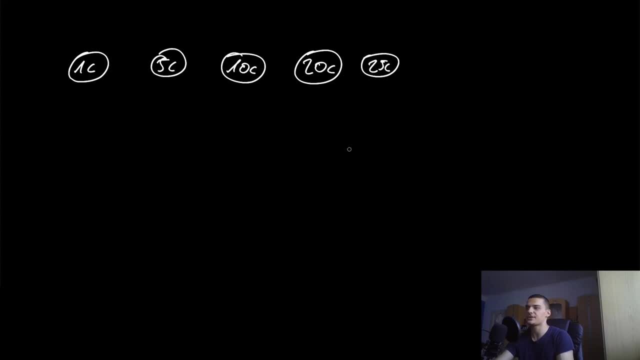 here. these are ordinary numbers and the goal now is to find optimal solutions. Now, of course, if I have something like 30 cents, I can go ahead and say: okay, 25 cents plus 5 cents is 30 cents, so I have two coins as the optimal value. So I can go ahead and say: okay, 25 cents plus 5 cents is 30 cents, so I have two coins as the optimal value. 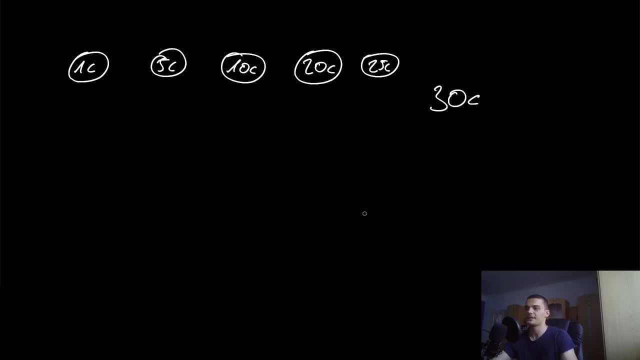 So sometimes it still works, but not necessarily every time. For example, let's look at 40 cents, and 40 cents is an example where this would not work, because the greedy algorithm asks: what is the coin that I can use to decrease this value the most? right now, The greedy algorithm is: 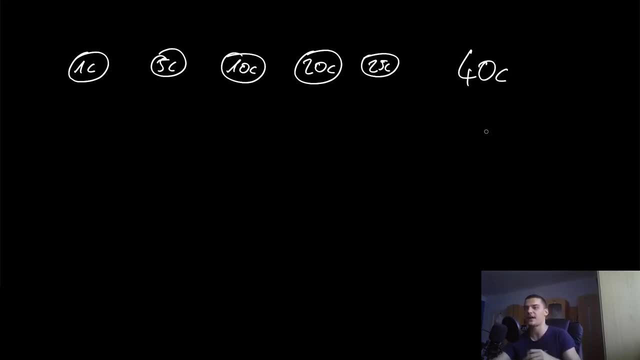 interested in the best solution locally. We want to decrease the value to zero. okay, the best solution to do that right now, as far as I can see, is subtracting 25 cents. So okay, we'll just go ahead and do that. What we do is we end up with 15 cents, then I go ahead, subtract ten cents. 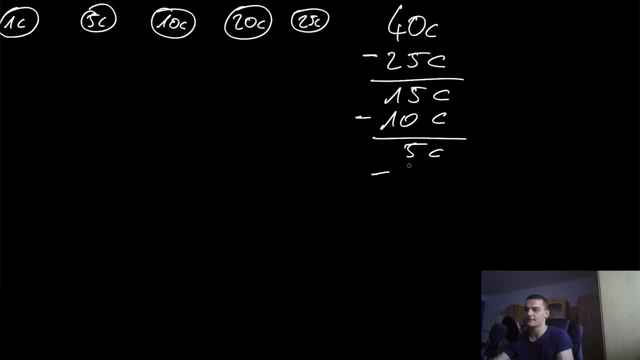 end up with five cents, and then we go ahead and subtract the five cents and we end up with zero cents using three coins. However, this is not the optimal solution, because the optimal solution is not a greedy solution. the optimal solution is just picking 20 cents. 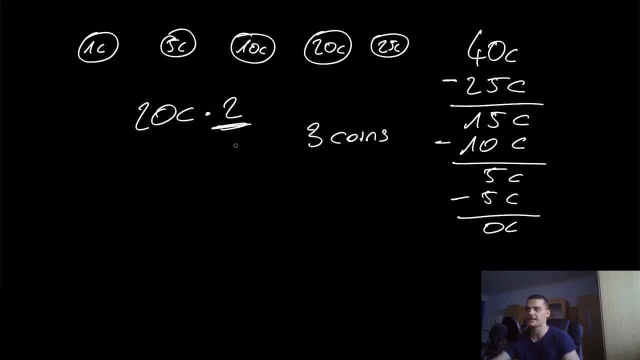 two times Two coins and we still end up with 40 cents. So this is, as you can see, a proof that greedy algorithms are not an optimal solution always, especially not in general, but also not for this example, where sometimes, in some constellation, a greedy algorithm always gives you the optimal. 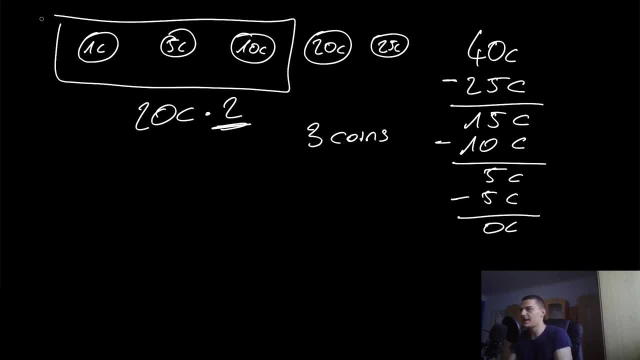 result. if you only use these three coins here, a greedy algorithm will always give you the optimal result. however, sometimes, in different constellations, it's not going to be the case, so you have to be careful, and I just want you to know what greedy algorithms are, that sometimes they work, sometimes they don't work, and